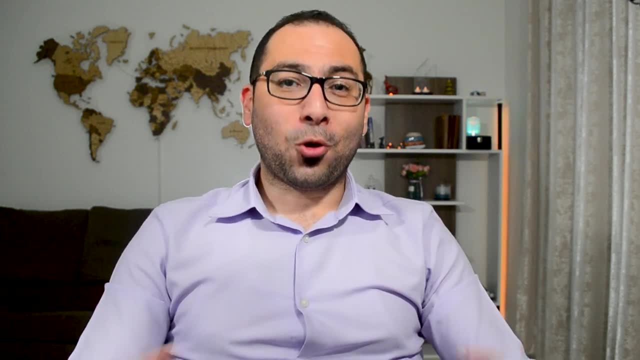 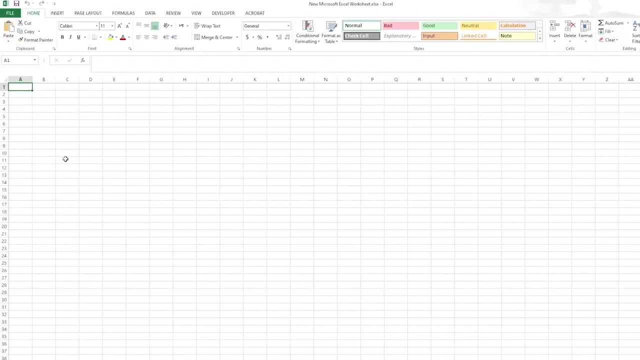 required skills and enhance your knowledge to elevate your cost engineering career. so if this is what you want, you know what to do. actually, this channel is for you and let's start. so i am here and i am having a blank excel file and let's see how can we make this. 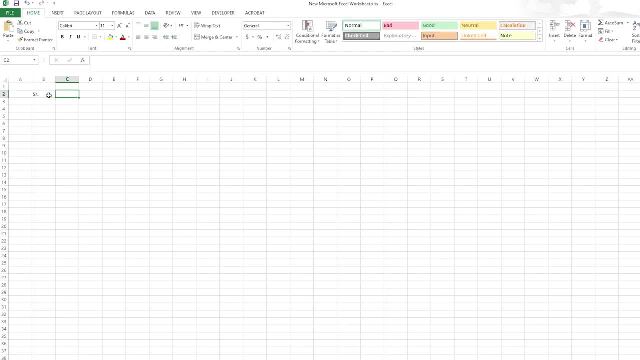 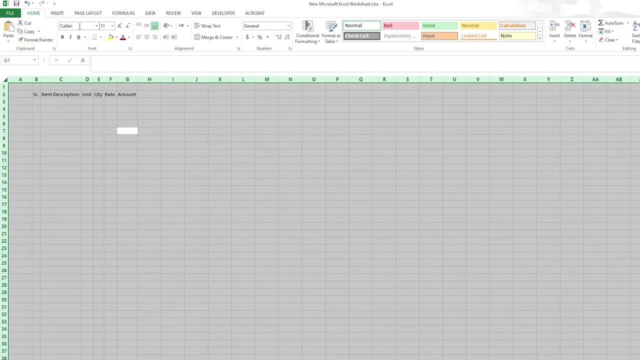 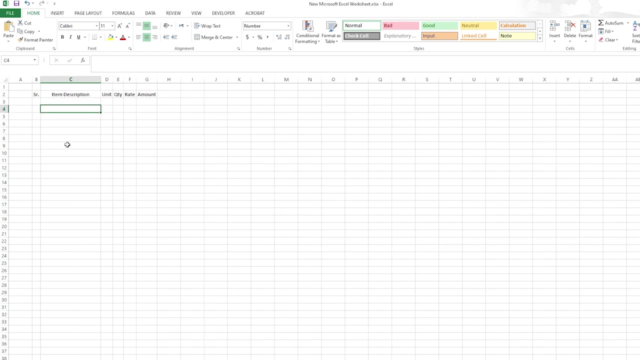 comparison. so i'll just start with a serial number and item description, then unit, quantity, rate and amount. and before i start let us just select everything here and we can make everything center and right click here and go to format cells, and i want all the cells to be numbers. so now let's start writing our items. let's assume that 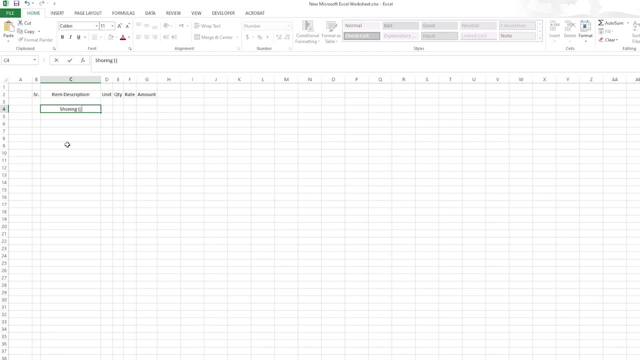 this is an enabling work package. so i have here shoring and let's assume, for example, this is second files and we have some type x and also we have the excavation and, let's say, leveling, and we have the second files and we have the excavation and we have the watering. 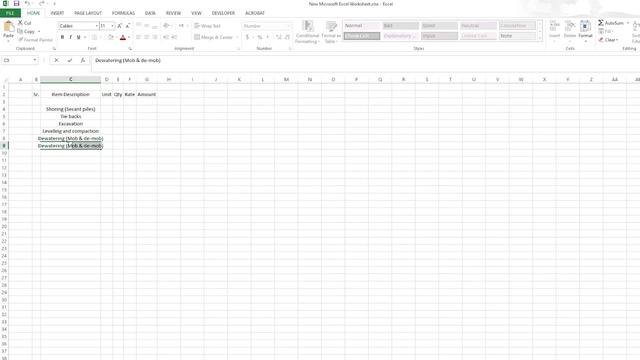 the watering. i'll have two things i'll have, let's say, first thing is mob and the mob, so mobilization and demobilization or removal of the system. and i have that, the watering. let's say i have the running. so I have the dewatering, mobilization and we have the running also. and these 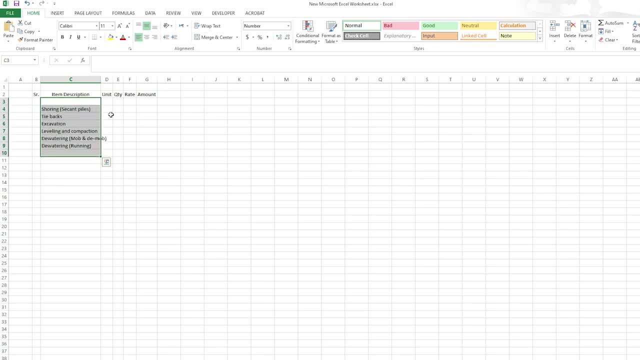 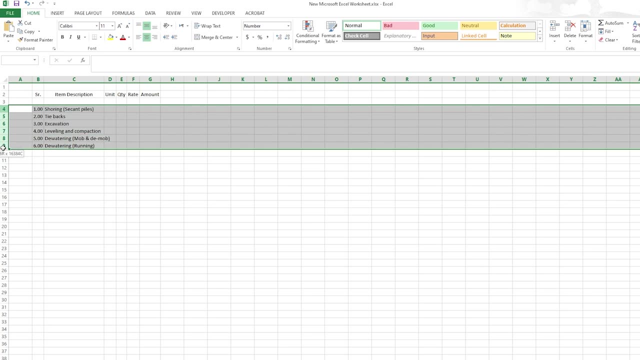 will be our items here. so I'll just make them start from the left like that, say one, two, three, four, five, six, and these are the six items that we have here for this comparison, and I can just select all of them like that and click ctrl plus to add rows, as you see, between them, and I can select this column and I'll 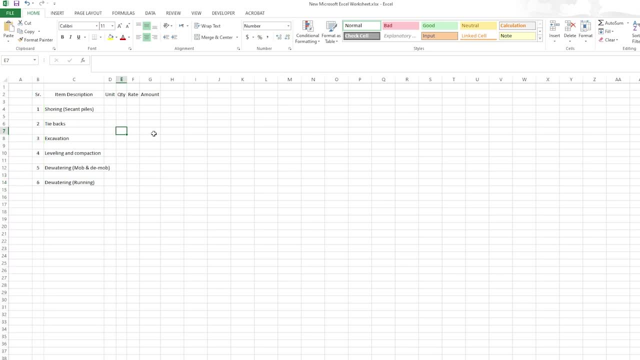 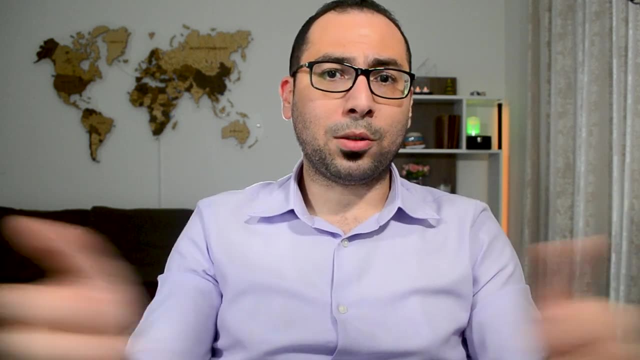 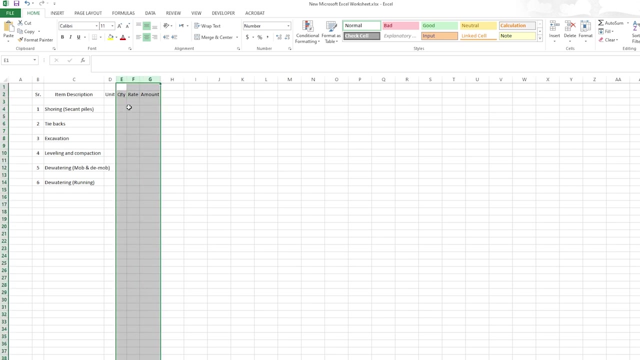 just decrease the decimals, so just one, two, three, up to six. and now let's assume that I have quotations from different vendors and I want to compare these quotations. so how to do that? let's go back to the screen here and, as you can see, quantity rate amount. this quantity rate amount will be from the first. 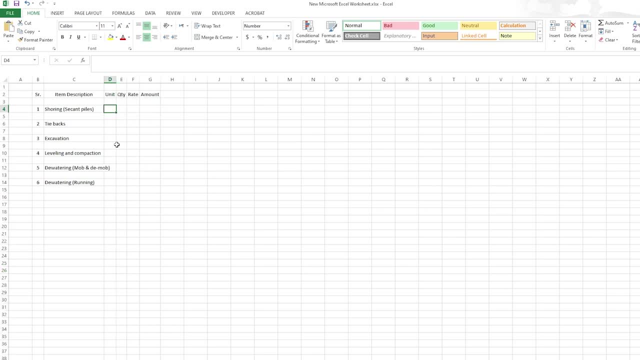 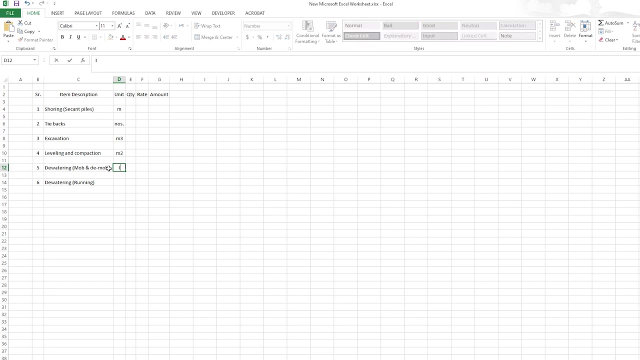 vendor. so let's put the unit of measurement first. so let's say, for example, the shoring will be in linear meter, the tie backs will be in numbers, the excavation will be in cubic meter, the leveling and compaction will be in square meter, and this will be like an 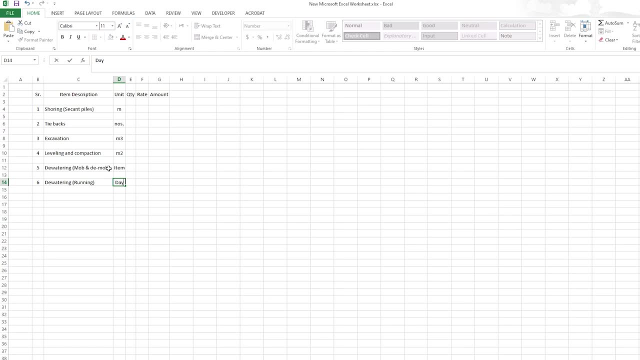 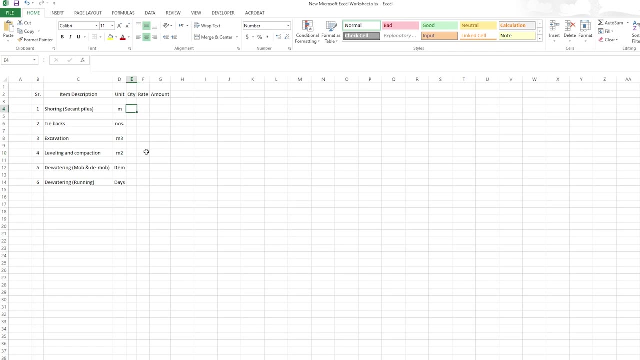 item and this will be in days. the running or the quantity of running the dewatering system will be in days. and from the first one let's say here: okay, let's just make this meter square, I'll just select it. then right-click format cells, superscript, so to have it look like that, and here same superscript. 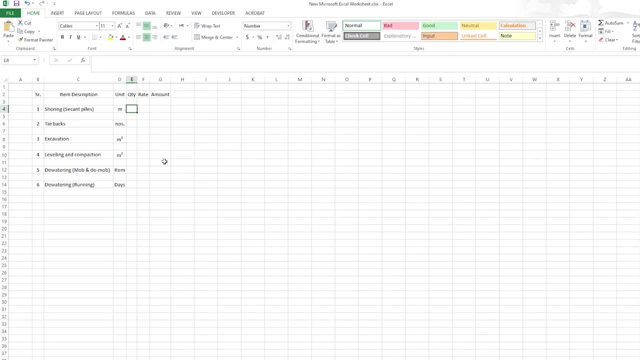 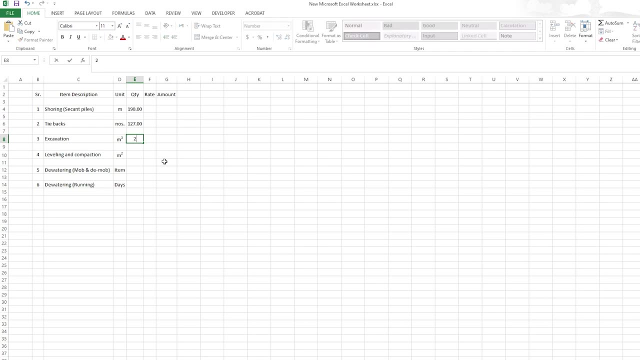 ok, so that's it. now. let's assume that we have 190 linear meters of shoring and 127 tie backs and 20,000 cubic meters of excavation, and let's say, 2200 square meters of leveling and compaction. the dewatering mob and demob will be one. 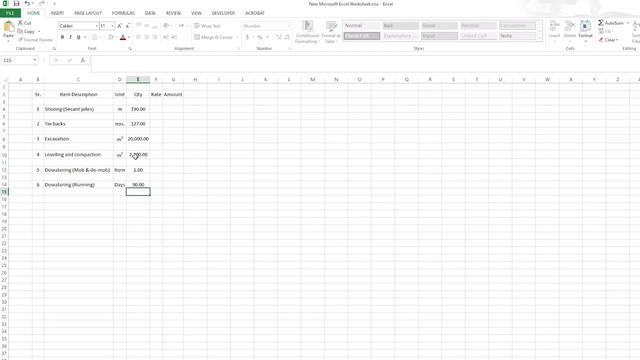 because it's an item, and let's assume I'll run the dewatering system for 90 days. now let's have the rates here that we got from the first vendor or first company. let's say here 11 500 and let's assume here 2000. 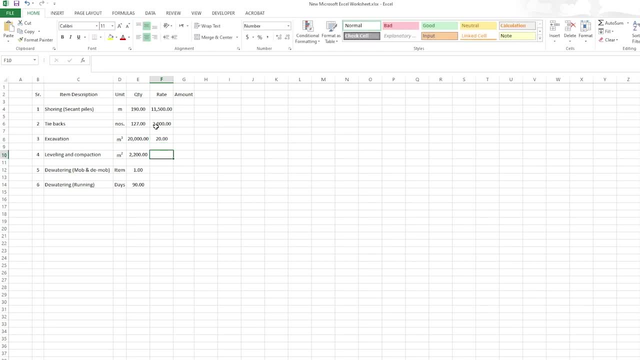 and here maybe 20, then 10 for the leveling and compaction, then maybe 15 000 for installation and the installation of the system and maybe here for the running, 1100 per day. so let's get an amount now, i'll say, equal to quantity multiplied by rate, and i'll just copy this formula and paste it here. 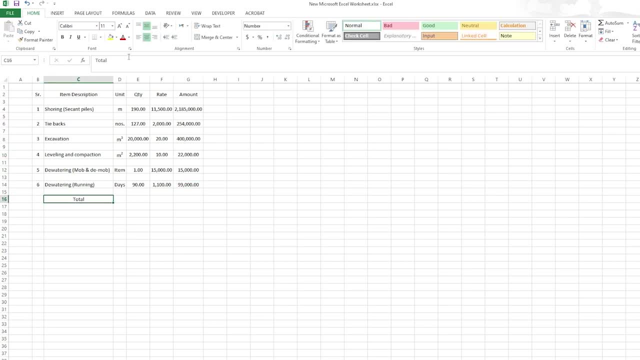 and let's have a total here. so this is the total for this vendor. the total will be this submission. let's take up to here, no problem, so 2.9 million. let's just do some quick formatting here. so i'll just mark that all borders and then i'll mark here: 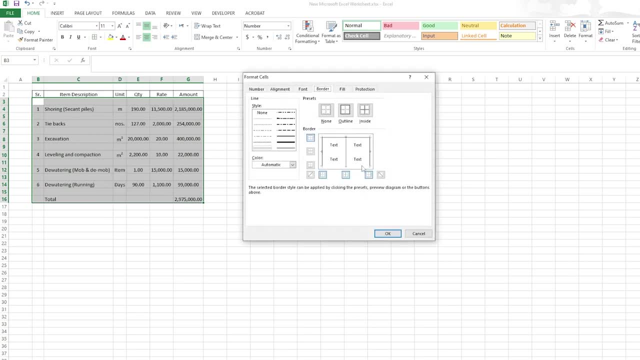 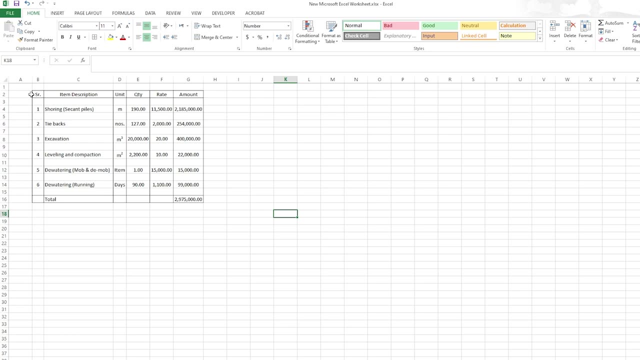 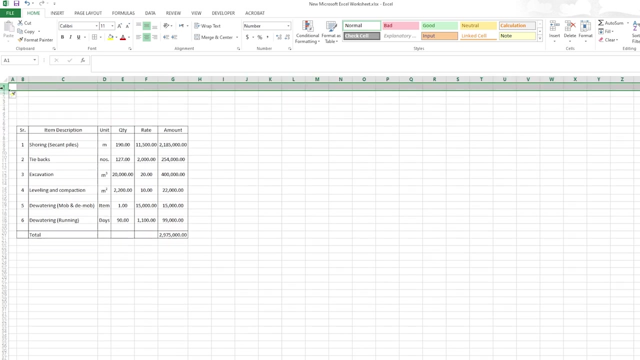 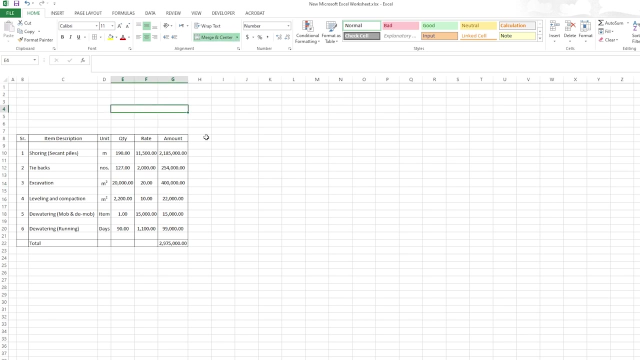 and i'll go for vertical ones and down, and then for the total i'll just select it and all borders. so i have something that looks like that. now let's add a few rows here and i'll tell you why now. so let's say that this is vendor number one. so here let's merge these cells and let's write: 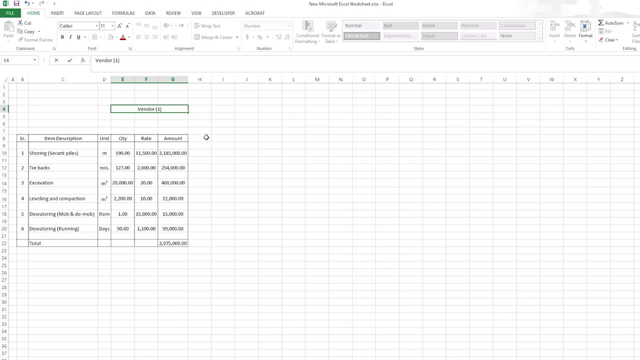 company name or vendor one or whatever, so vendor one. then here we can put the contact person and his mobile number, like jaune or whatever name, then the number. after that let's have here the quotation reference, because any quotation from a vendor will have a reference. so this is the reference number. 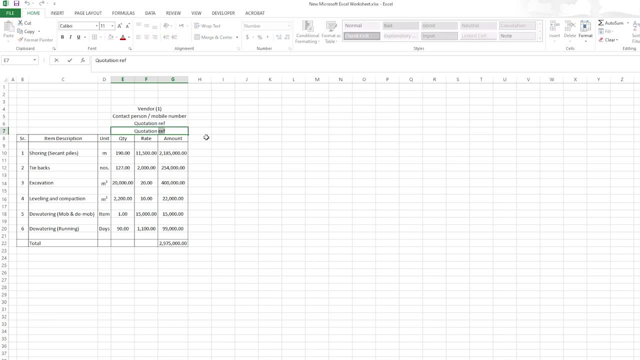 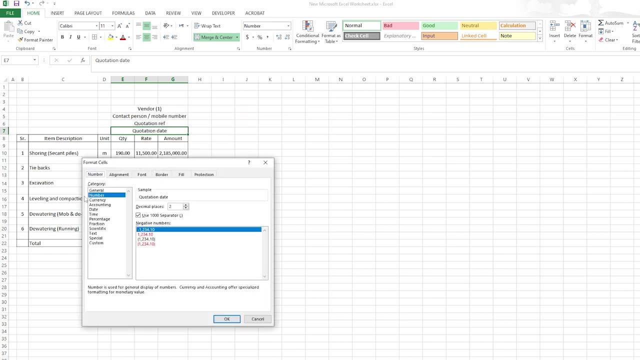 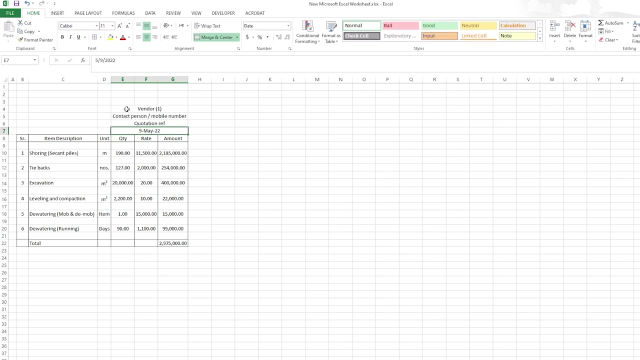 and here i can have the quotation date. quotation date actually for this one. let's right click format cells and go here and change it to date and choose this format: 14 march 12, for example, something like that. so, for example, if i say 19 may 2022 and i'll just select all of this and i'll make it all border, 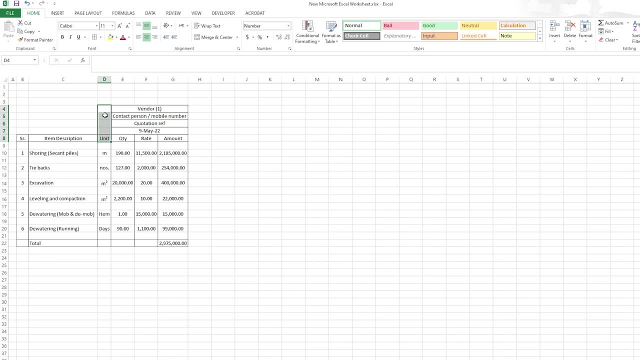 and now i have here i can go and merge all of that. but actually here i can put, like i can say vendor, here and here i can say contact, here i can say reference and here i can say date, because once you fill this information you will have here only the information. so you need to know. 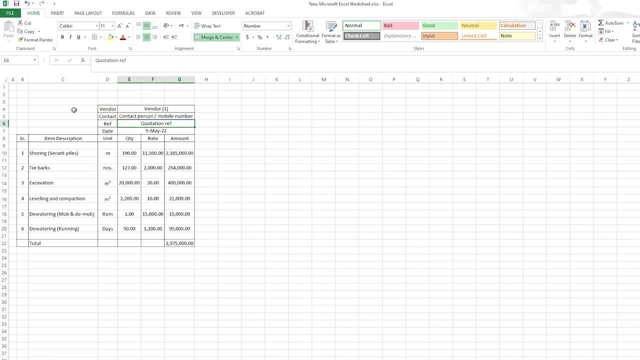 this information are for what? so we can add this part here. and for the description we can make all these cells together. and for the serial number we can do the same and then just select them and do more borders. so i have something that looks like that, that Now if I copy vendor one and I paste here, I can have here vendor two. 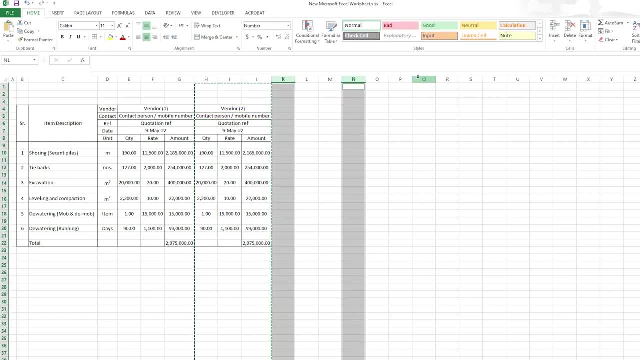 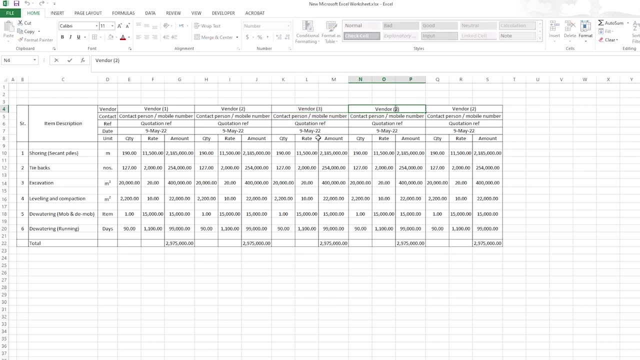 And if I copy this so I can paste here and here and here, for example, so I have five vendors, I'll just change the numbers or the company name: three, four, five, And of course, from the quotations from each of these ones I'll just update the price. 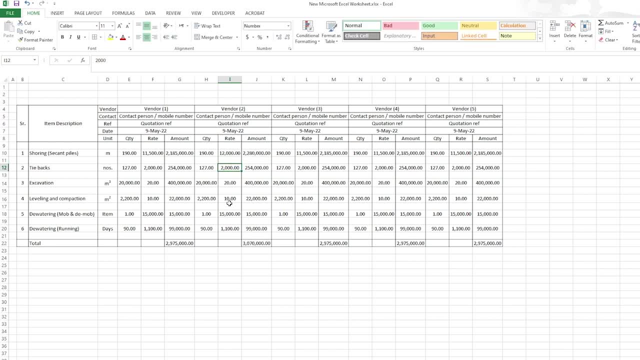 So let's assume that I have twelve thousand here, and let's say one thousand seven hundred fifty here, And let's say the excavation is twenty five, leveling and compaction fifteen, And let's assume this one twelve, And here I have one thousand five hundred. 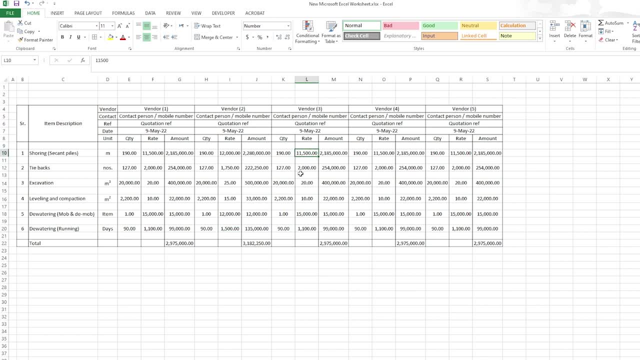 It's a different quotation. And here also let's say for example, ten thousand, And here tiebacks let's say two thousand, five hundred, excavation. let's say eighteen, And then here maybe Something like sixteen, and then or let's make it twelve, and then here let's say twelve. 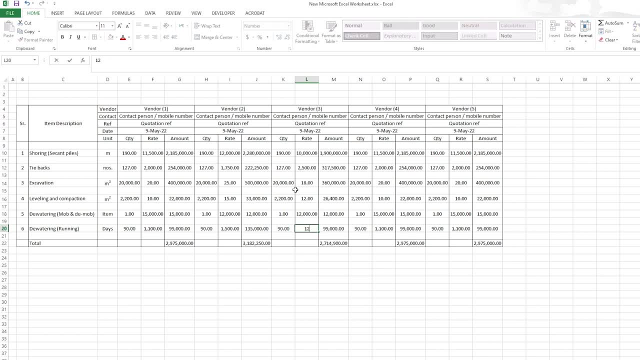 also twelve thousand, and here let's say one thousand two hundred. So each vendor is just giving his price Or his rate. Let's go for this one, and let's assume that he has given us here twelve thousand five hundred, and here let's say one thousand six hundred fifty. and then 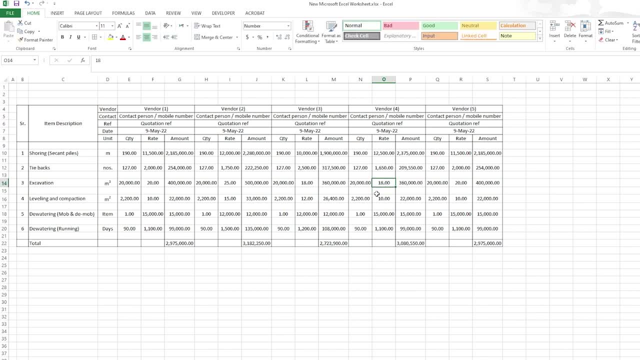 excavation, let's assume eighteen, or we used eighteen already, So let's go for seventeen. leveling and compaction: Let's say twelve, and let's see here, not twelve, We used it. So let's go for eleven thousand, and let's say one thousand three hundred fifty. 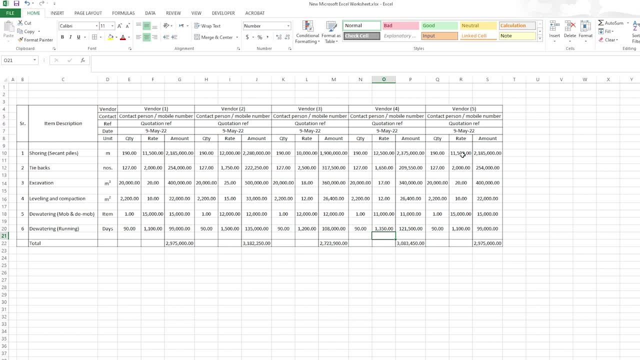 So this is another vendor that we have here and vendor number five. Let's just delete it. Let's keep it only for vendors for now. to make it simple, So for each vendor, I have quantity, rate, amount, and I can see something that looks like this: 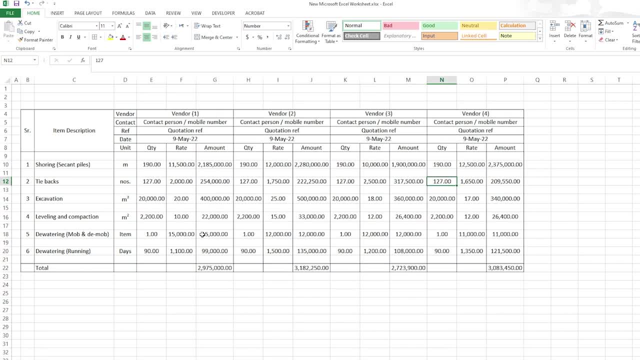 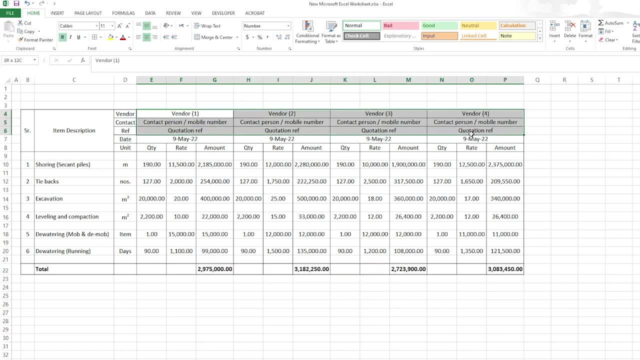 I'll just zoom in a little bit to show you what else we can have here. So first thing, I'll just make this bold and also this information- We can have them bold, including the quantity rate amount for each of them and similarly this: 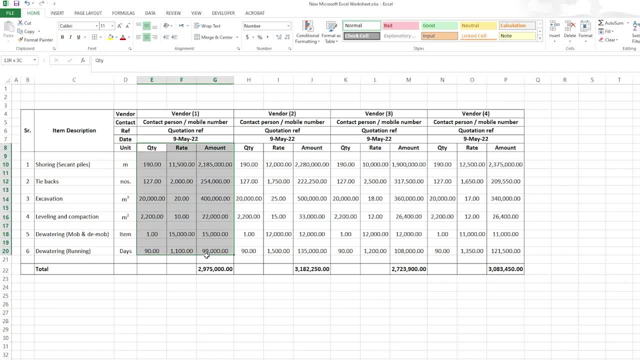 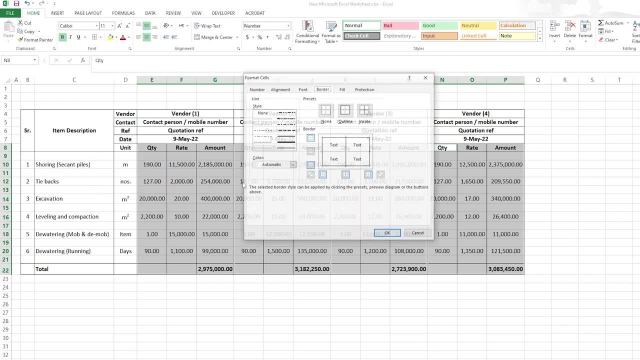 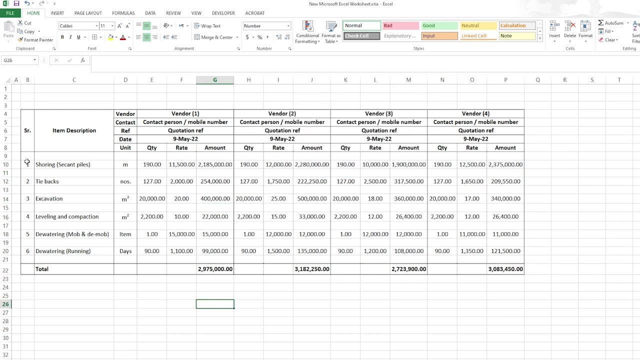 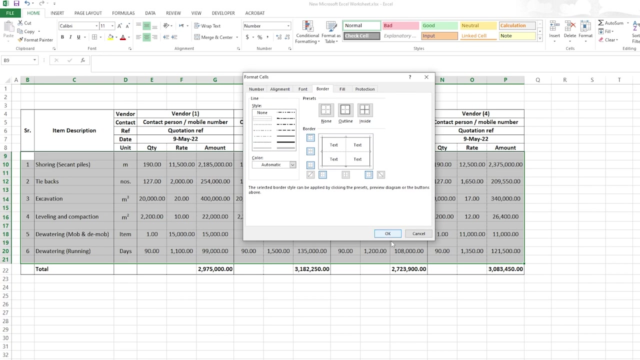 information And actually inside here. if you select them like this one by one and you go to more borders, you can make the Inner one as a line that is dotted, so it looks like that much better And we can have here. also, if you go again to more border, I'll go dot it for the horizontal line so it can. 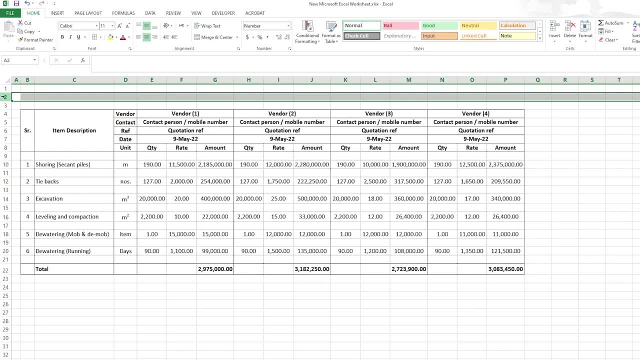 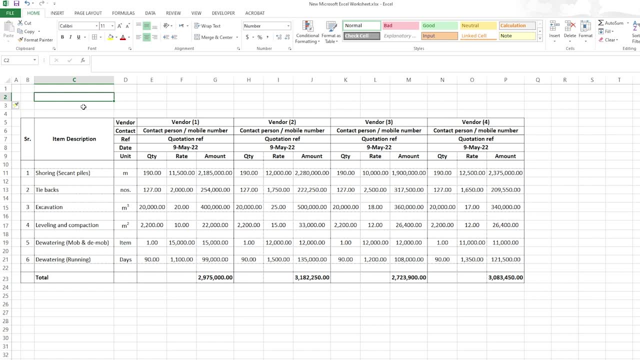 look like that, And here I want to write some information related to this project. So, for example, I can have here something like your company name, maybe company name, And then We have. We can have, let's say, procurement department or contracts department, depending on who is doing this comparison here. 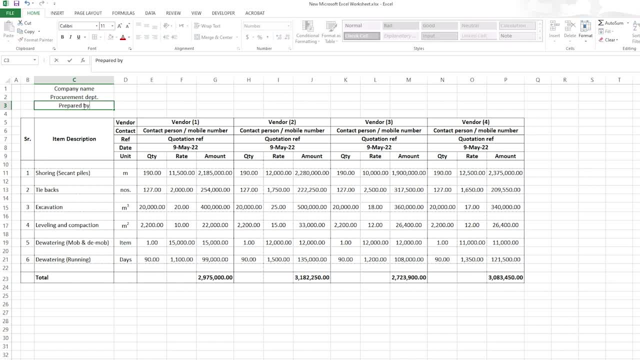 You can have something like prepared by. in that case it will be a model, for example: And that's fine, no need for more. So I have these things. Let's add one row up and make them start from the left, like that, and then I can go. 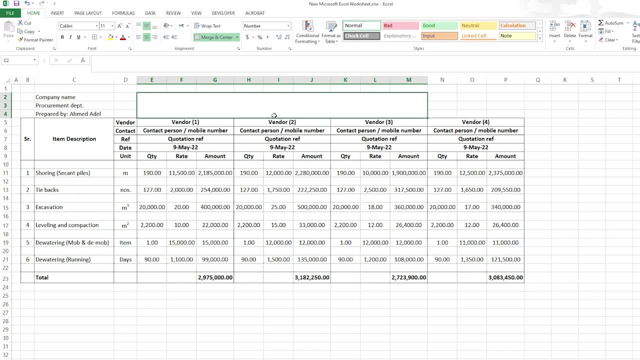 And I can merge these cells here, something like this, and I can say, for example: quotation or price comparison sheet For Enabling works, And I can put here the project name And actually That The Row. 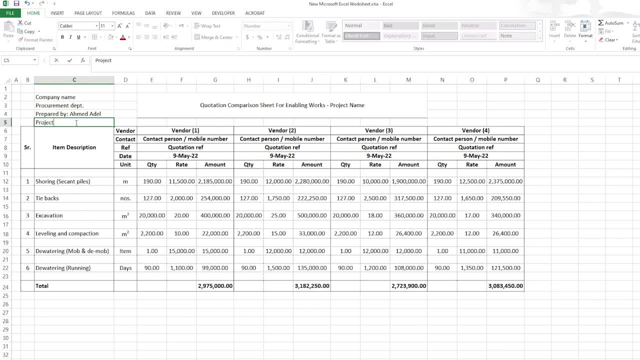 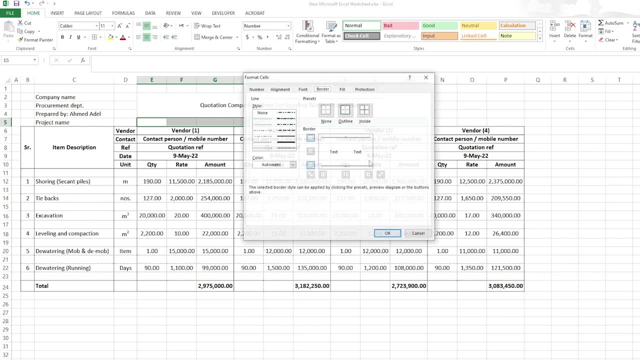 That I Delete it just now. you can have the project need name here also. so I am doing a comparison for this particular project and this line. I don't want it, so I just go to more borders and remove it like that and you can remove the merge and merge it again. 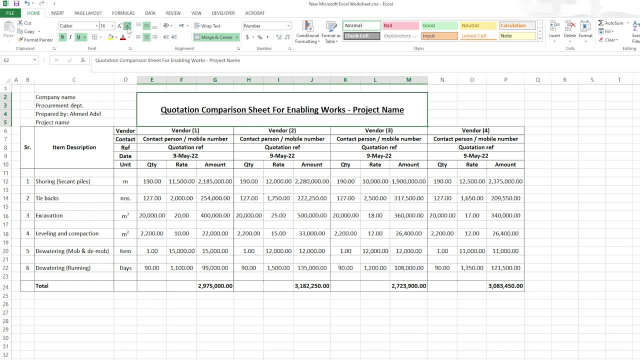 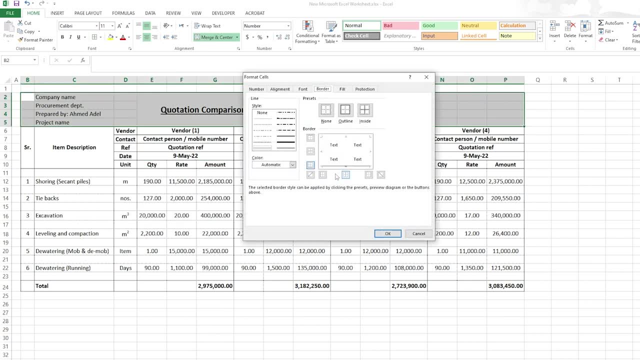 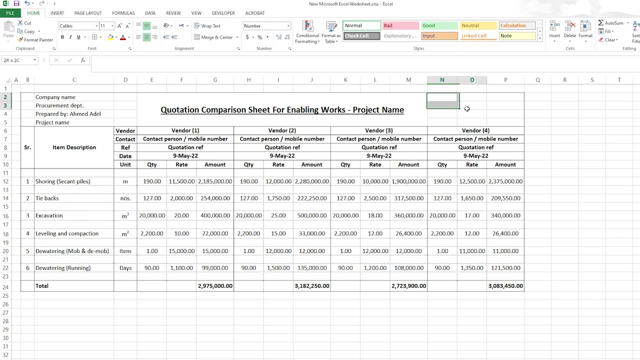 You can make this bold and underline and you can increase the font here. So if I just go and make external borders From Outside like that- OK, so it looks like this- then here I can make a border on the left side and I can merge. why? 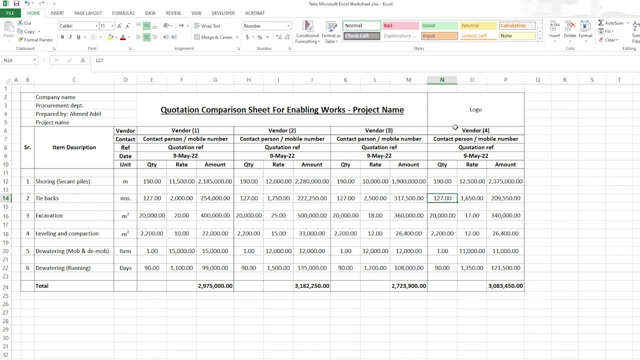 Because I can use this for putting the logo of the company. so you can put a logo here. You can insert a logo and put it in this area, but it is very big, something like that can be OK. so you can put the logo of your company here. here you can write this and we will. 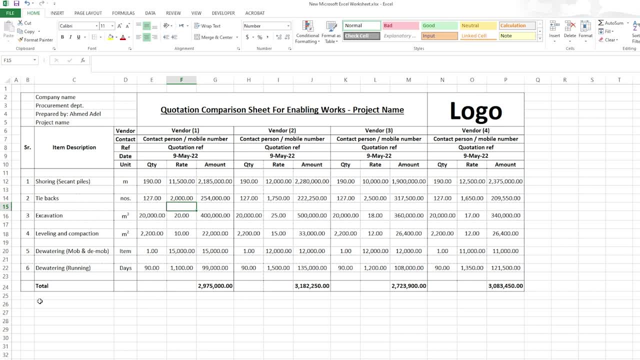 Have something like that. OK then, and down here I can have, for example, let's say, duration or delivery time or something like, And also, other than the duration, we have the terms of payment. So I'll put here terms of payment. 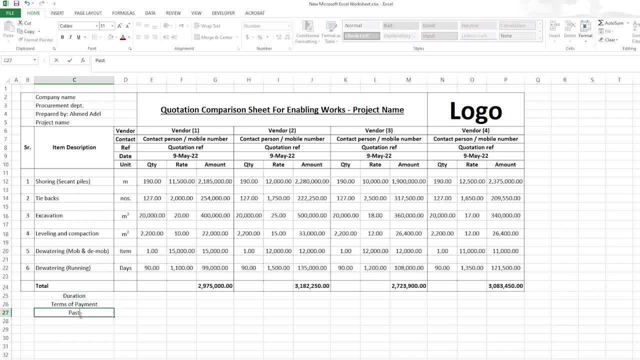 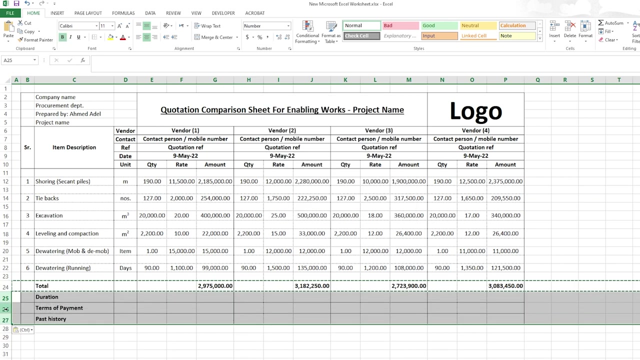 And we can also have, let's say, Past history or Like, for each of these vendors. So First, what was our past history? Did we deal with him before? Good experience, bad experience, and so on. And We can copy the same formatting actually. so I can copy this line and I'll paste the formatting here, like that: 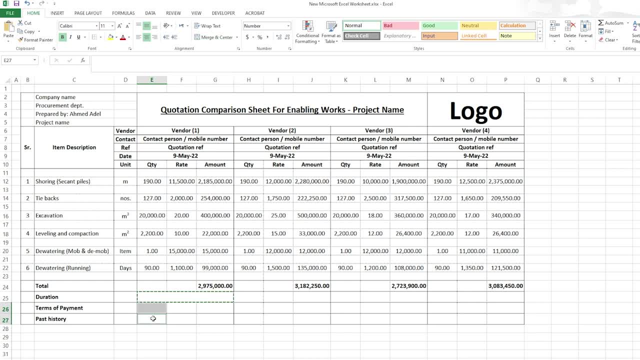 And let's merge this and copy it and paste it here and here. So I have three merged cells here. Let's copy them and do this here and here and here as well. So let's say, for example, that the duration here or the duration offered by this vendor is 90 days, and here also let's say 90 days or 100. 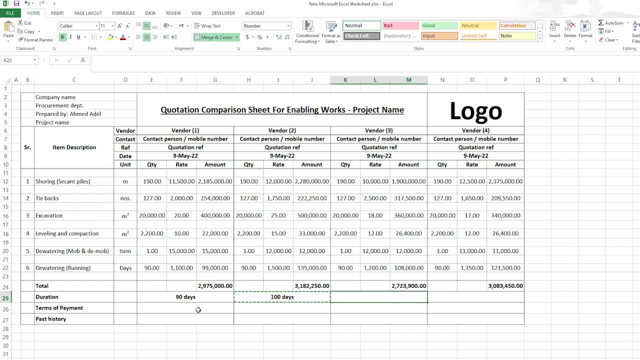 Let's make them just different. And this one is offering, let's say, 100 days as well, And the last one is offering 90 days also. And the terms of payment: let's say here: 30 days BDC, for example. 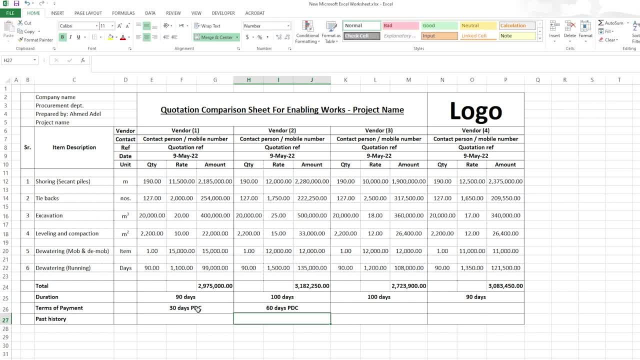 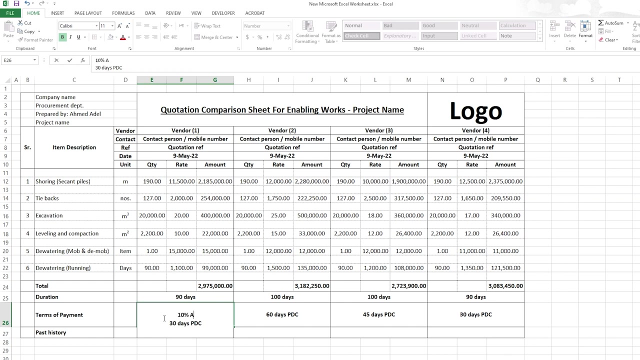 And let's say here 60 days. OK, let's say here 45 days, and here also let's say 30, and let's assume that all of them are asking for an advance payment. so i can just write here: let's say: 10 percent advance payment. 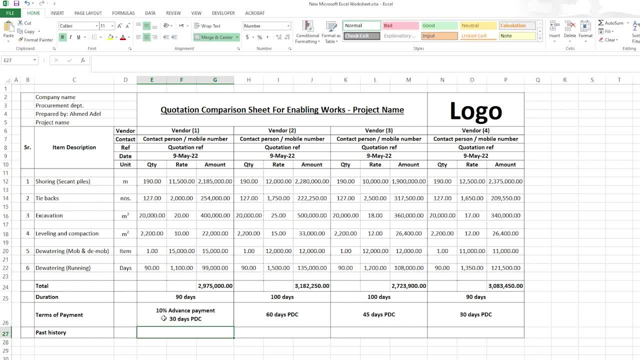 something like that. i'll copy it and here also: let's just bring this down and let's here say: this one is asking for 15 advance, and maybe here say 20, and this one is asking for 10 or 15, doesn't matter. so you can keep them centered like that, or, if you want, you can make them start from the left. 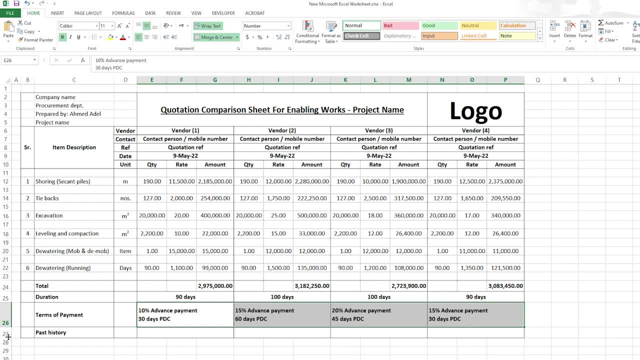 up to you. it's just okay, leave them like this and then here for the past history. let's say good performance, or performance. let's say here, normal, or, or, or whatever. let's keep them all good performance. so we are not looking into this. so let's keep them all good performance. so we are not looking into this. so we are not looking into this. 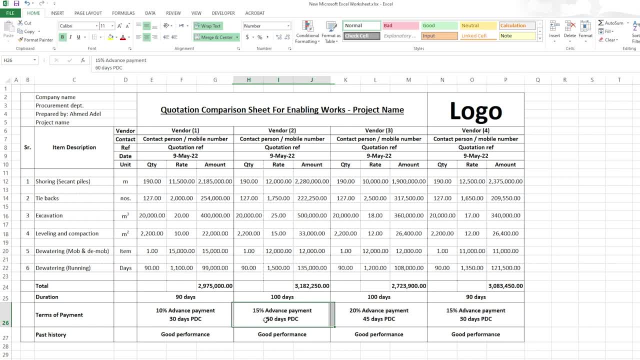 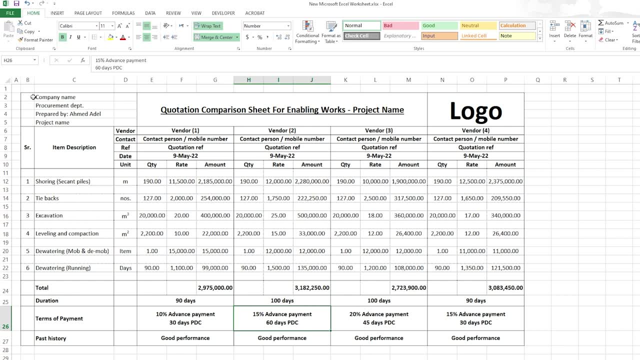 because all of them performed well in the past. let's have this centered so we can have something that looks like that: if you want to do some coloring, you also can. this part also. if we make it bold, it will look much better. and now let's go to. let's click ctrl p or press ctrl p. 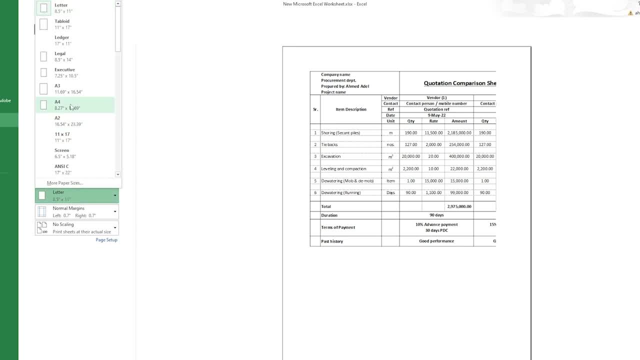 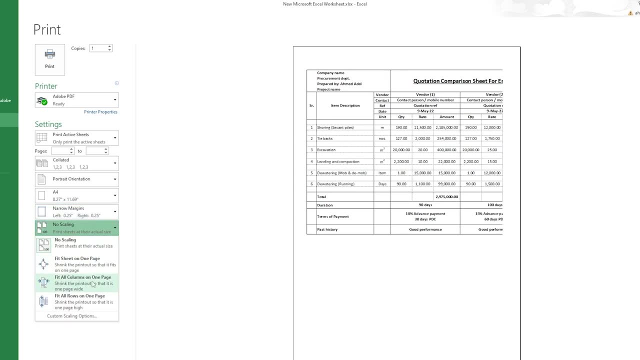 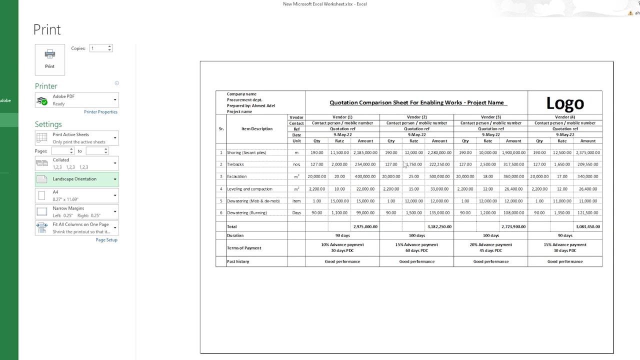 to see how it looks. so let's from here, from the paper, let's use, for example, a4, and for the margins let's go for narrow. for the scaling let's go for fit all columns in one page, and for the portrait orientation let's have it landscape, so it looks like that when you print it will look something. 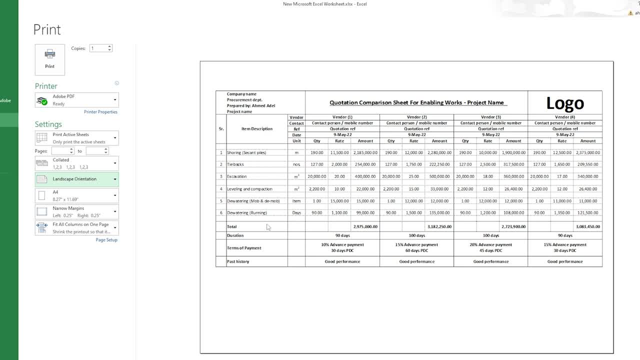 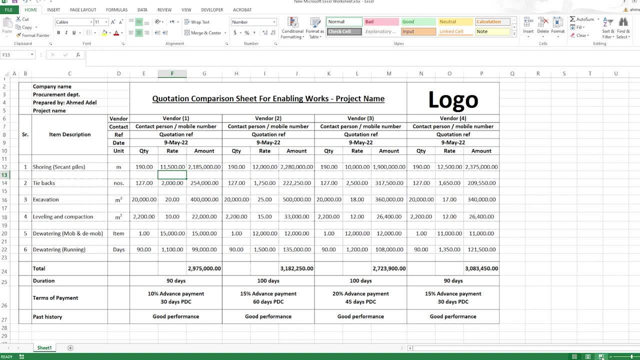 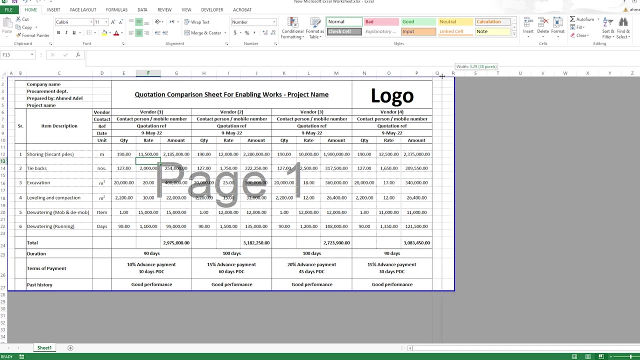 like that. if you wanted to take the full paper, let's say, then i'll skip this. and here you can see here beige breakdown preview. if i click that, you see, so i can just bring this to the left a little bit and decrease this one, and i can bring this down and let's reduce. 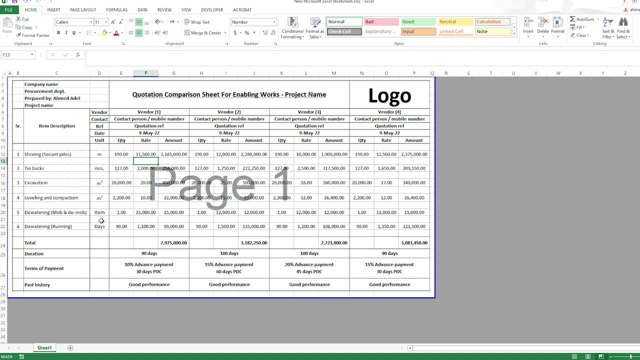 the size here a little bit now. i'm just trying to make it more beautiful looking. and let's say here currency, for example. you can put it here and you can say here: total amount, just knowing now doing the final touches for this. so if i want to make it give it more height, 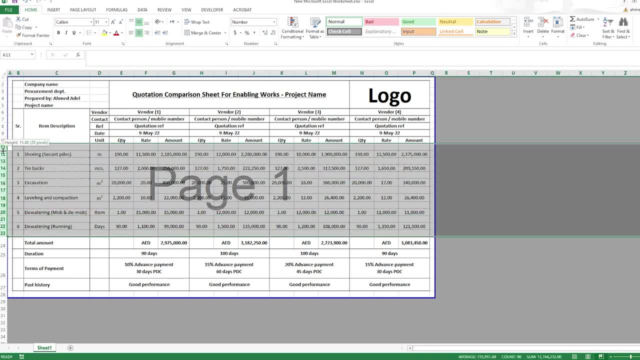 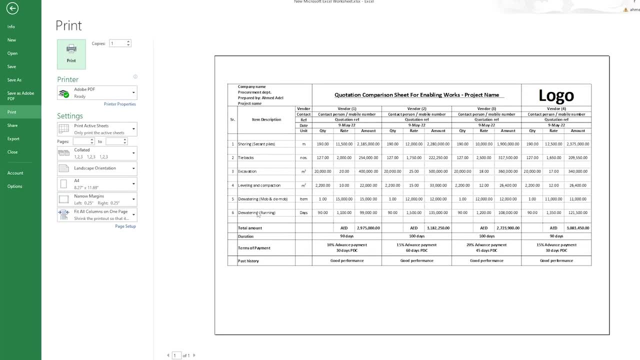 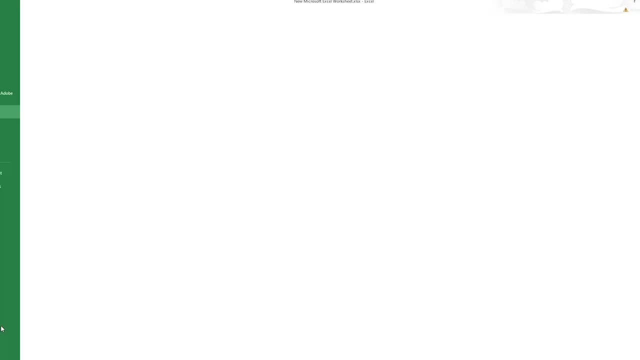 i can do. i can mark these rows here and increase one of them a little bit, so all of them will be increased like that. so if we print now, you see it increased. also we can increase the duration a little bit. terms of payment- past history. i just wanted to fill the paper so it can look nice of. 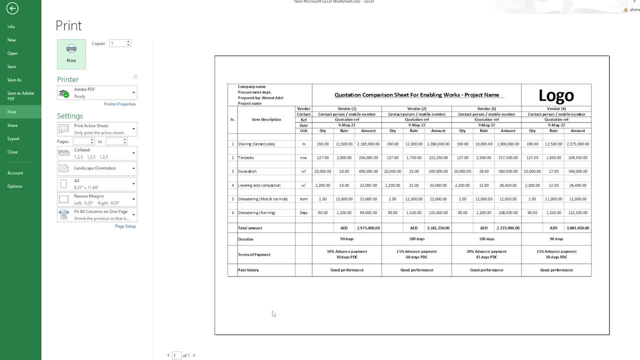 course you can put here people who will be signing on this comparison sheet or something like. so you can have here like prepared by a checkbox, by final approval by, and people can sign on this paper and based on that you can award or make a contract or something like that. so that's it for this video. thank you so much for watching and i 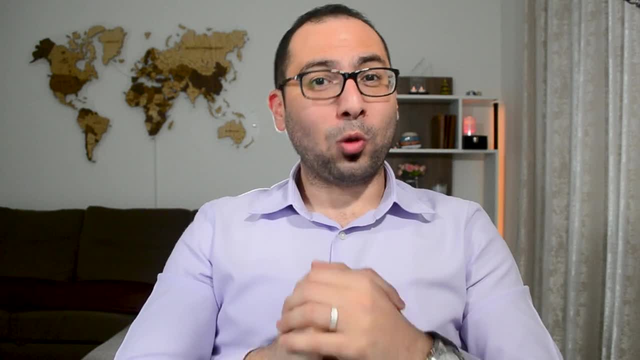 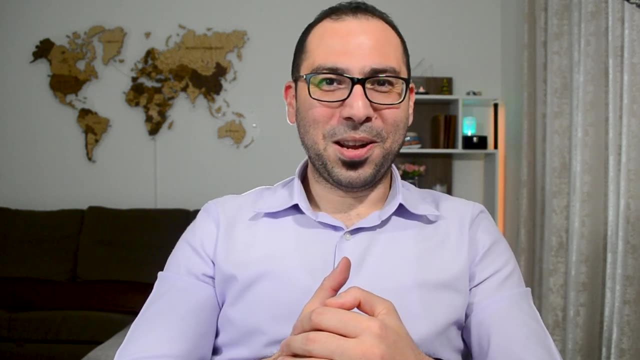 appreciate your valuable time. if you have enjoyed this video, don't forget to like and subscribe to the channel and give me a comment in the comment section down below, and see you in the next video. bye, bye, you. 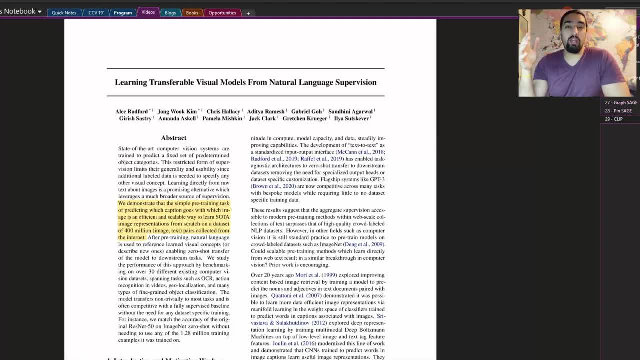 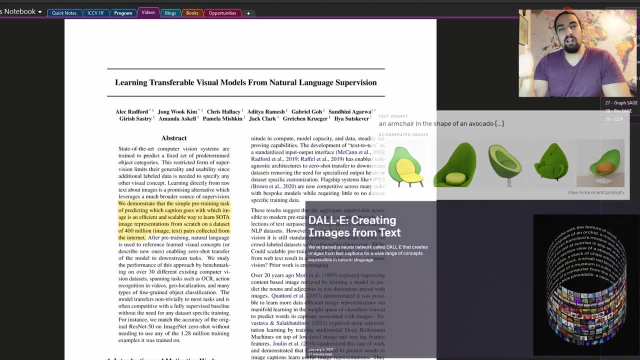 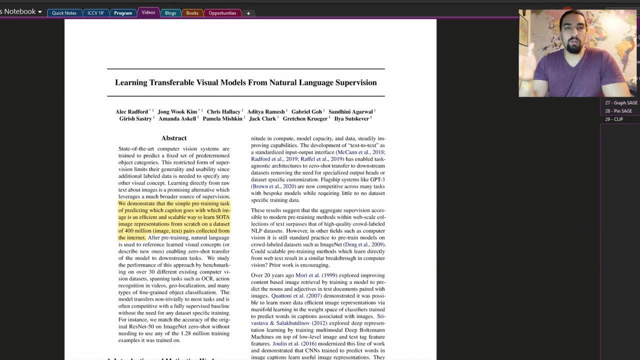 Hi there. So a couple of days ago, OpenAI published two really exciting research works and among them DALI took pretty much all of the media attention and was all the hype. but I found this work, CLIP, or Learning, Transferable Visual Models from Natural Language Supervision. 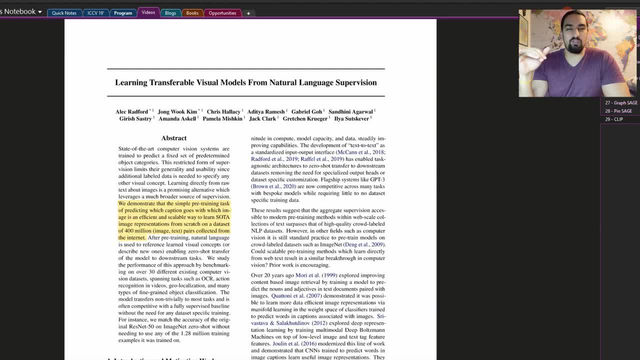 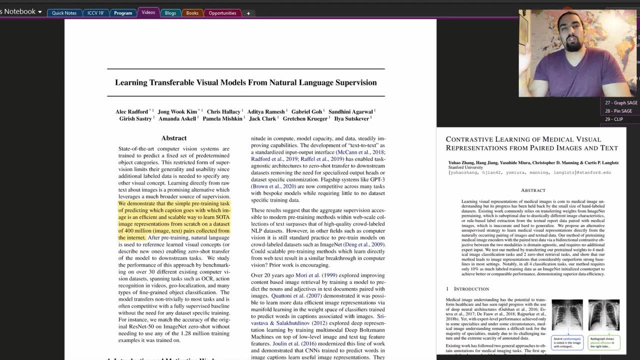 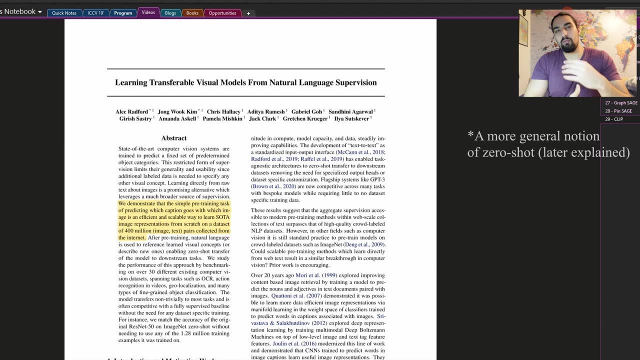 really exciting and I want to cover it in this video. So basically, the method itself is not new, so it's just a modified version of Convert paper. but the thing they introduced here is a concept of using zero-shot in computer vision. 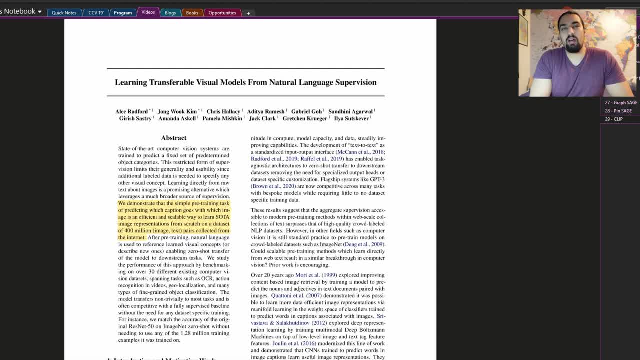 So they're probably not the first ones, but they are really bullish on it. It's pretty much a continuation of their exploration of the GPT and all of the zero-shot capabilities it had, and they're now trying to take that NLP parallelism.